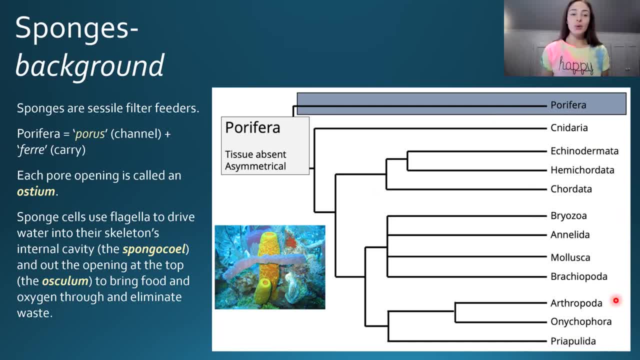 we're just going to be talking about porphyra or sponges, And so porphyra, to give a little bit of context behind that name, because it sounds kind of weird. for sponge it just comes from porous and that's why they're called porphyra, And if you think about sponges that makes a lot of sense. 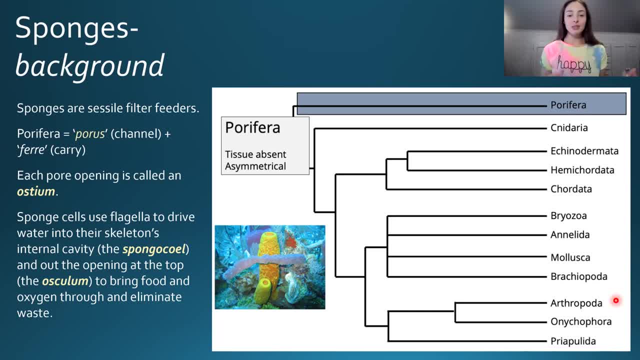 They're super porous And their pores have openings called ostiums. So now jumping right in and they have cells, which we'll get into more specifically what each cell type is called in a sponge on the next slide. But in general their cells use flagella to drive in water into their 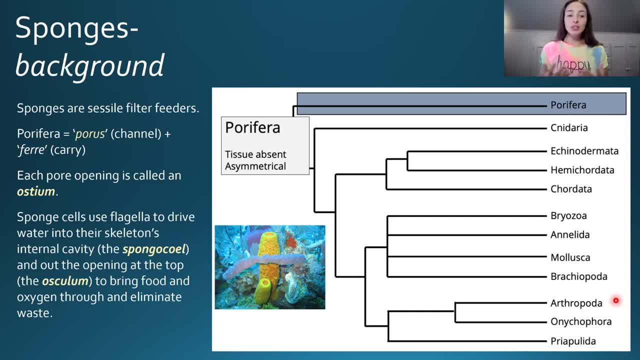 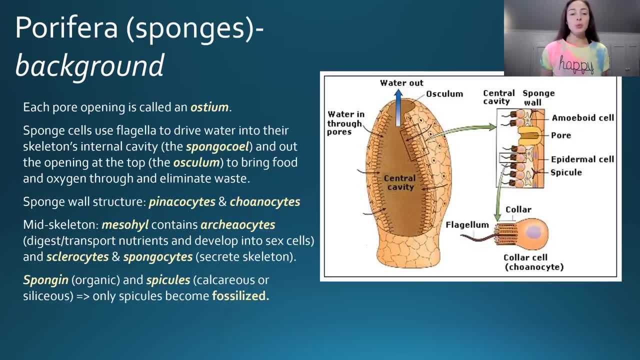 internal skeletal cavity called the spongicle and out the opening at the top or their osculum, And this is to bring food and oxygen in and eliminate waste, And so they're filter feeders. In more detail, their body structure looks like this: As we can see, the ostia or pore openings are shown. 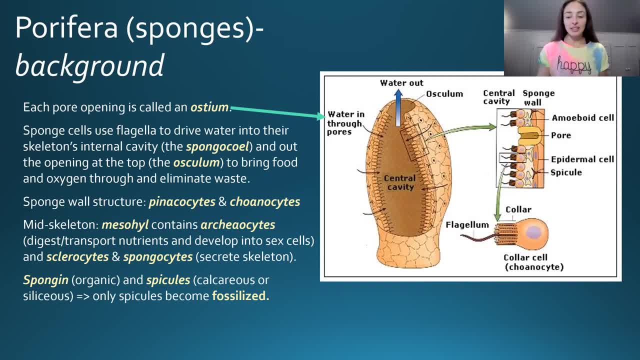 here to bring water through and into the spongicle, Our central cavity shown here, And then we have the osculum at the top, which is the opening where the water goes out, eliminating waste, And then we have different types of cells, shown in the. 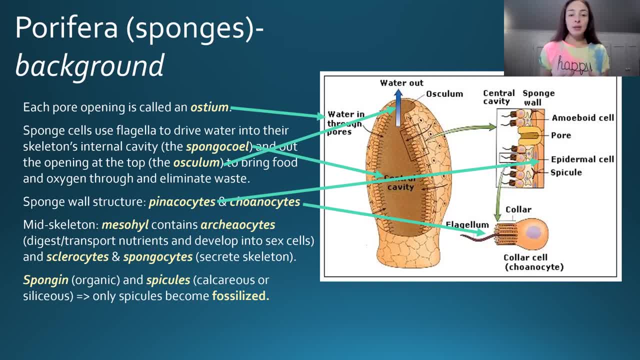 zoomed-in figures to the right in this image, And what these are are pinnacle sites labeled as epidermal cells, shown in the figure on top, And then at the bottom figure there's a zoomed-in image of a choanocyte, And these have the flagella that help with the propelling and filtering of the 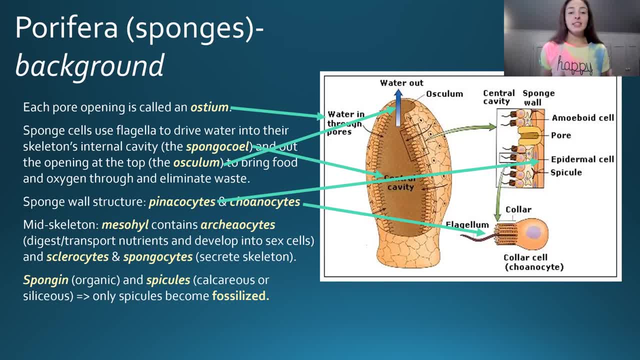 water, And then they have a mid-skeleton called a mesohill, And this contains archaeocytes which digest food, transport nutrients and eventually develop into sex cells, And it also contains sclerocytes and spongocytes which secrete the skeleton And you. 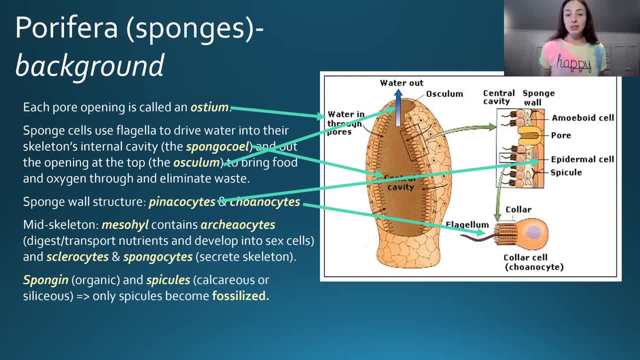 might not be thinking that sponges have skeletons, but they do, And sometimes they're made up of an organic protein called spongin, And sometimes they're made up of spicules, which can be made up of calcium carbonate, in which case they're calcareous, or silicon dioxide, or quartz, in which 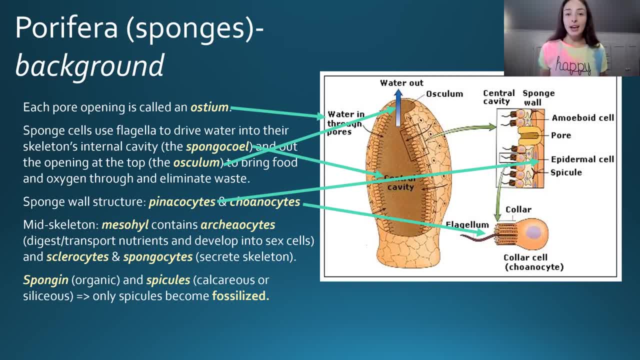 case, they're siliceous And a lot of times, sponges have both of those things, And they're also made up of spongin and spicules, And this helps support their structure. However, in terms of paleontology, 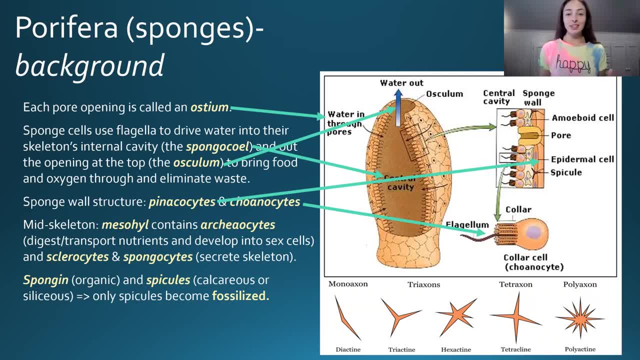 we'll be focusing mostly on the spicules, And this is because these are what get preserved. Because spicules mineralize into calcite and silica. these hard parts are what's going to get preserved And unfortunately that makes it hard to decipher the fossil record of sponges, sometimes because 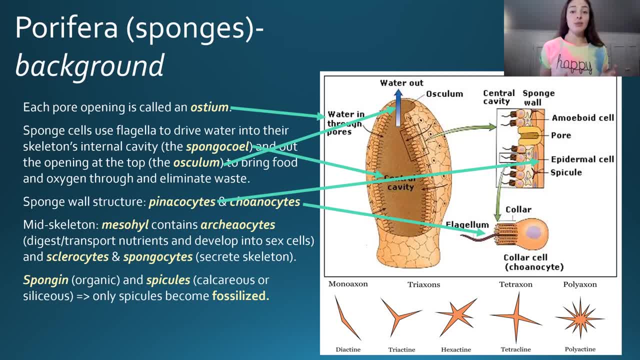 sometimes it's just a bunch of spicules that aren't actually in their original sponge structure anymore And they're just spread out in sand grains and whatnot. So that's unfortunate, But sometimes they're still congealed into their sponge structure And the type of spicule matters in terms. 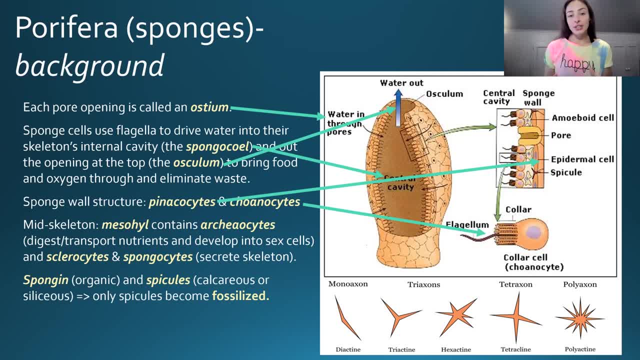 of interpretation of type of sponge. So if we look at the bottom figure here now, we can see types of sponge spicules. These include, but are not limited to, monaxone, triaxones, tetraaxones and polyaxones. 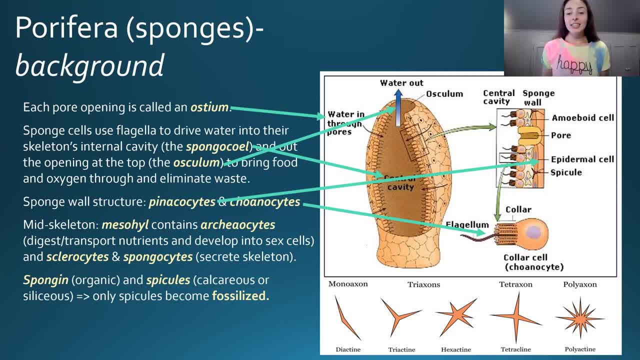 And these, more specifically, can be called diactene, triactene, hexactene, tetractene and polyactene respectively, And sometimes these sponge spicule types can take on different morphologies, but still within their 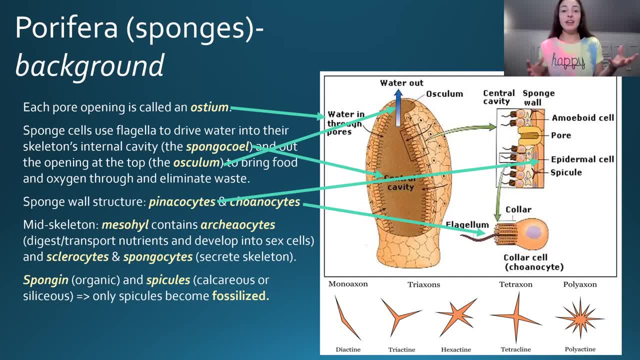 spicule class. So, for example, you might have a triaxone that has one longer ray than the other two rays, or a tetraaxone with a similar type of longer ray than the others. So all of these slight nuances and the differences in the spicule morphology, as long as they're consistent within 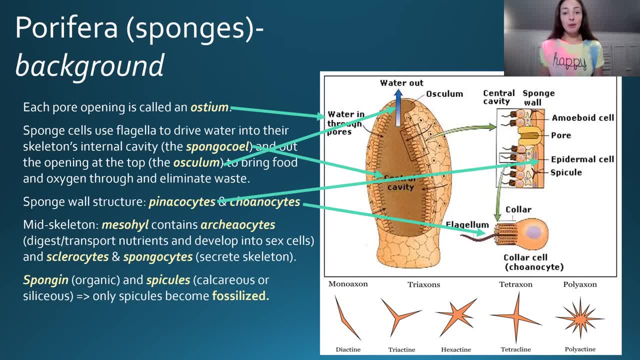 the sponge specimen you're looking at can tell you a lot about what type of sponge you're looking at in terms of the broader class, as well as more specific differences in the spicule morphology. And so later, when we talk about different classes of sponges and their types of spicules, as well as their 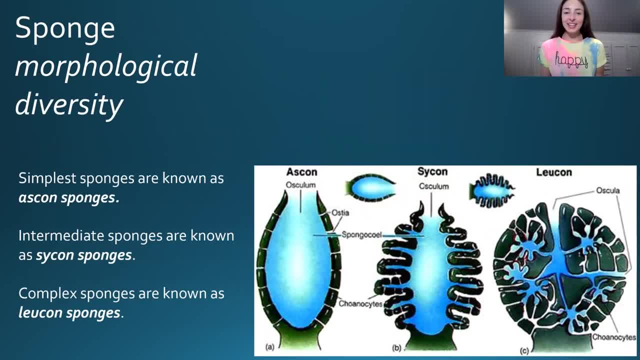 structures and other characteristics. we'll talk about these again, But before we get to that, we have to talk a little bit about the differences in simple versus complex sponges. Now, these aren't necessarily taxonomic groups of sponges, but these are categories of sponges based on complexity. What we have here 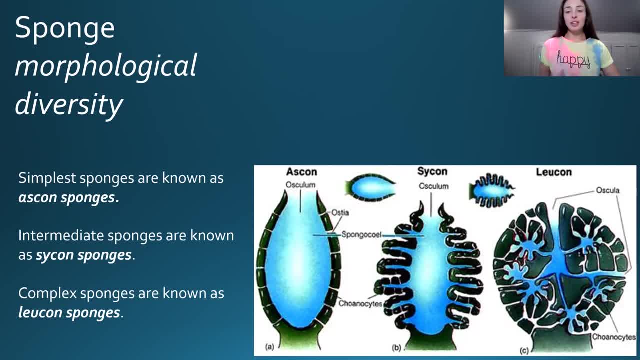 are three groups: Ascon sponges, Cycon sponges and Lucon sponges. Ascon sponges represent the simplest morphological structure a sponge could have. Ascon sponges have an osculum ostia, a spongicle and choanocytes, just like all of the main structures we already 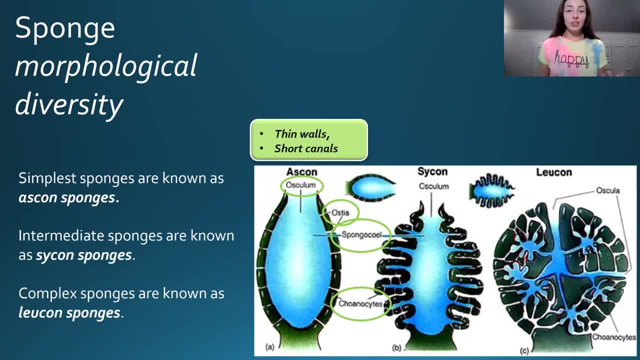 discussed. But their simplicity comes with their walls which are thin and their canals which are short. As we can see, with the Cycon and Lucon sponges we can see major folding going on, especially in this circled area of the Cycon sponge, And these folds are called incurrent. 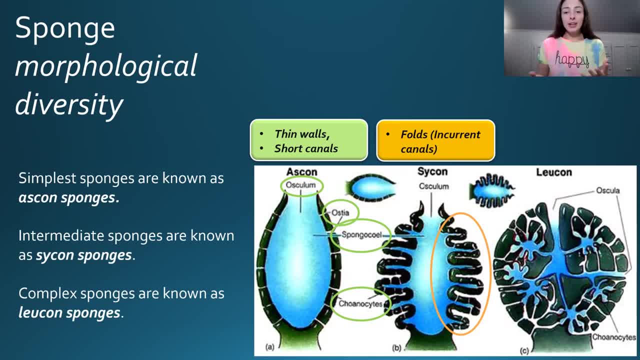 canals. These canals help to propel water into the sponges and they're called incurrent canals. Ascon sponges have a more complex design than the simple Ascon morphology. Lastly, we have Lucon, which we can already see is pretty crazy complex, And with this we see that it not only has an 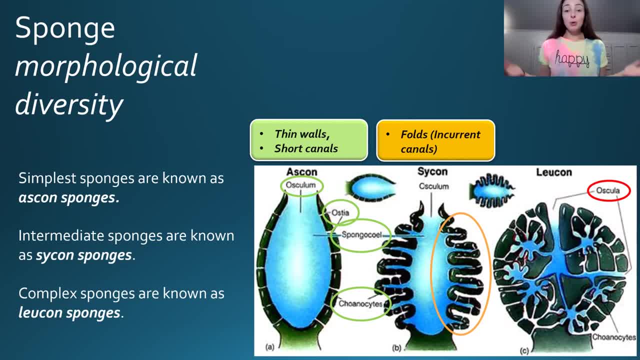 osculum but it has multiple oscula. It has multiple pore canals, like all the types of sponges, but it also has multiple out openings. Ascon sponges have a more complex design than the oscula, which none of the other types of sponges have. Additionally, it has this crazy squiggly. 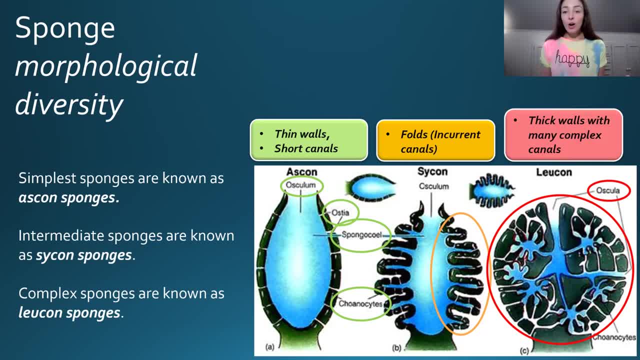 structure going on. And what's happening there is it just has really thick walls with many complex channels, And all of these channels have special functions to help propel water in and out of the sponge, to help it filter feed. However, in the case of Lucons, sometimes they can have relatively 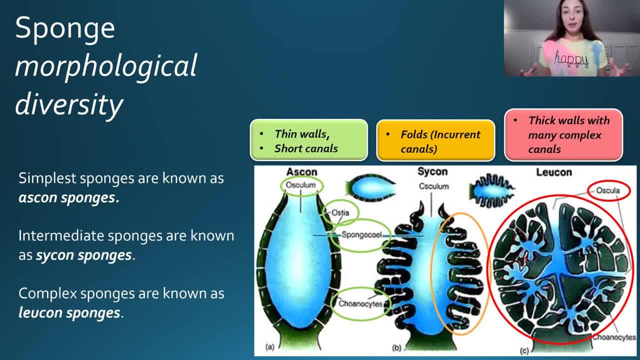 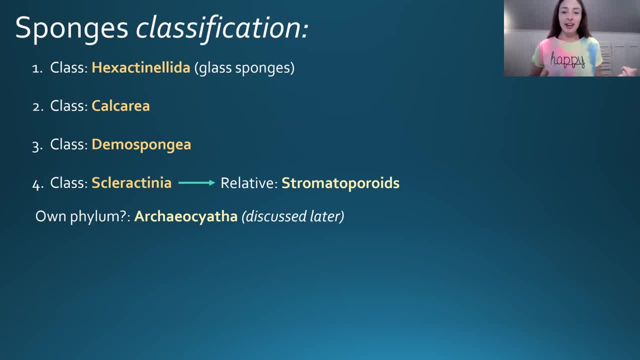 small spongicles or their internal cavity because of their complex, thick wall structure. And all of these things we've discussed so far are leading up to us determine what kind of sponge we're looking at when we're looking at a fossilized sponge. 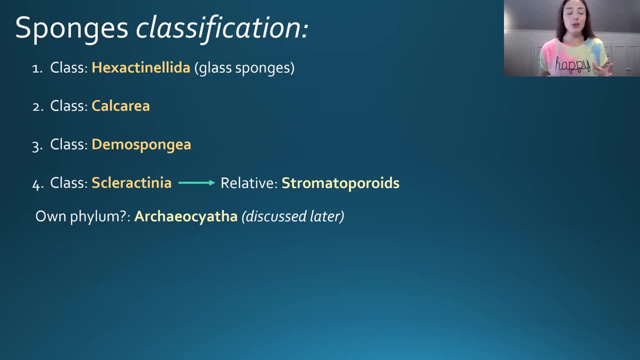 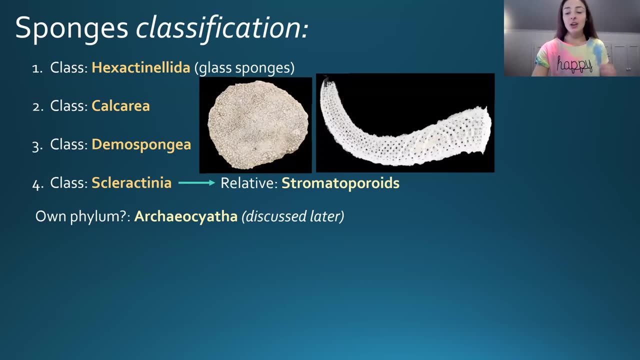 or fossilized fragments of sponges. So, to go over the major classes of sponges, we have hexactinilida, or glass sponges, we have calcarea, we have demospongia and we have. I just realized that. 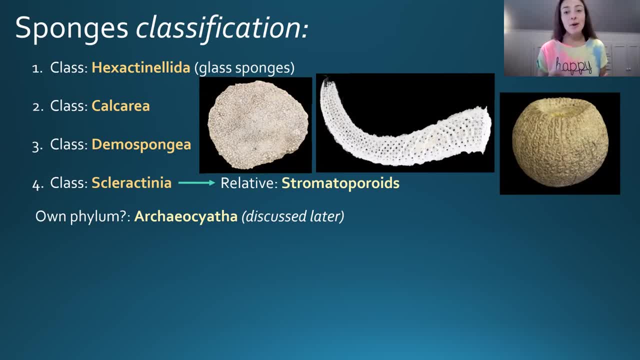 that says scleractinia, which is a class of corals, not sponges. This is a lesson to you out there watching this, thinking I know a lot of things. That's actually supposed to say sclerospongia, And because I'm too lazy to say sclerospongia, I'm going to say sclerospongia. And because I'm too lazy, 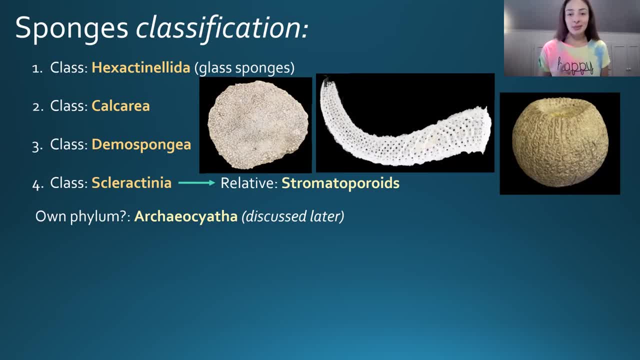 to change it right now, which I could do, but I'm not. I am going to tell you about it. So I'm telling you. I told you: consider yourself total sclerospongia. All right, moving on, I don't actually have a. 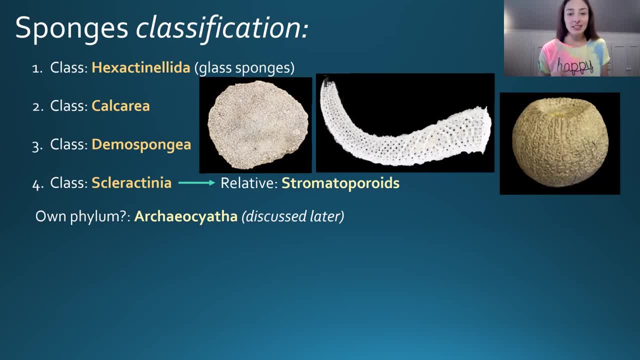 picture here of sclerospongia. Well, I guess, depending on how you class stromatoporoids, which could either be included in sclerospongia or a distant extinct relative of sclerospongia, or not even in the sponge phylum altogether, I don't know. We'll talk about why its taxonomy is so. 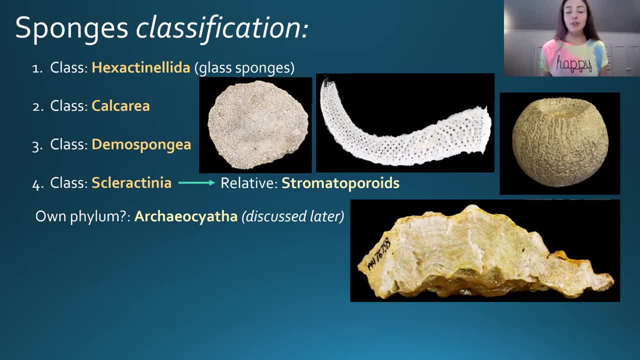 controversial later. But basically, I have here a picture of stromatoporoids and this is because these are what we're going to talk about later. This is because these are what we're going to be focusing on. These are the most important. 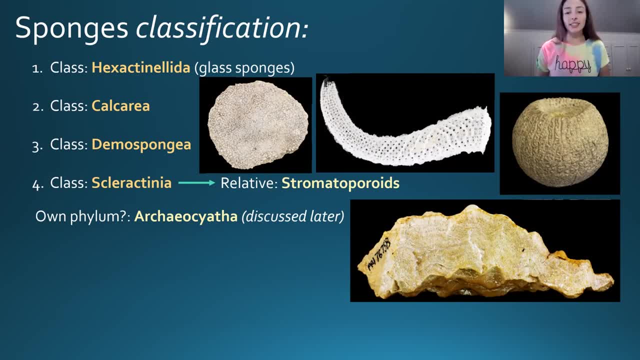 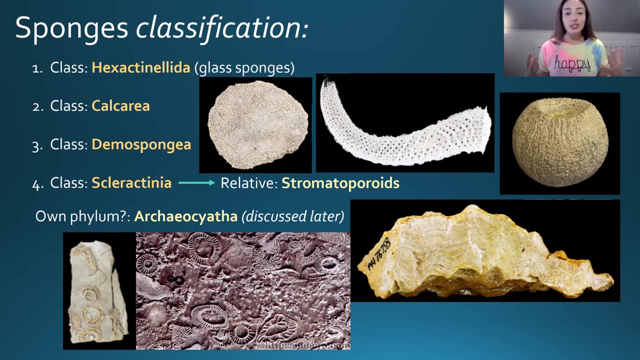 similar sponge, or maybe sponge to that class, and are very helpful fossils in ways I'll explain later. And then, lastly, another very taxonomically controversial group is the Archaeosciathans. These include some of the most geographically widespread and short time-ranged index fossils. 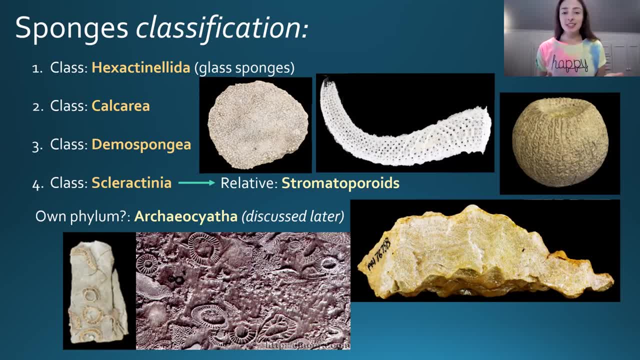 that you'll ever see, And so they're really, really important. However, we're going to discuss their crazy controversy in terms of their taxonomy and then we're going to talk about their classification and all of their characteristics at the end of the lecture, because they are not. 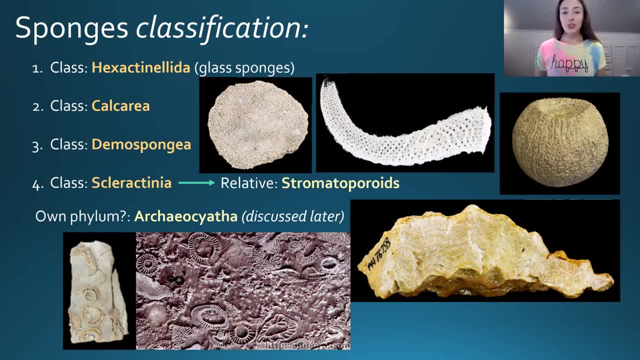 really technically confirmed to be part of Periphera. so they're kind of their own thing, And we'll talk about why paleontologists came to that conclusion when we talk about all of their other characteristics at the end of this video. But before that let's get into each one of the classes we just listed. 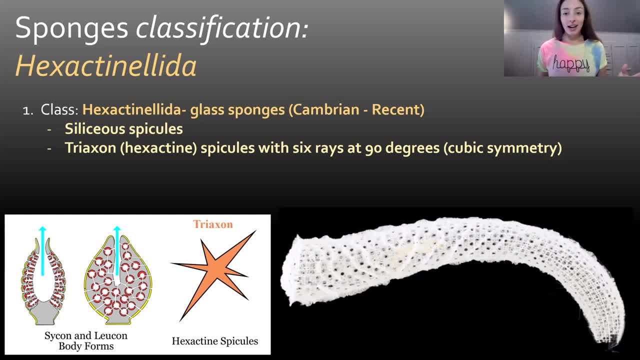 for Periphera We have the hexactanilids, which, like we said, are glass sponges. So what does this mean? This just means they have siliceous spicules. We talked about spicules either. 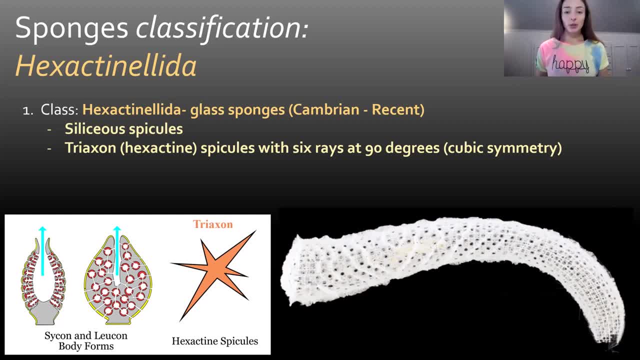 being silica or calcite, and these sponges have silica spicules, which is the same composition as glass, which means that their nickname glass sponges is pretty apt. Also, their time range was from the Cambrian to the recent or now, and then they have triaxon or hexactine spicules with 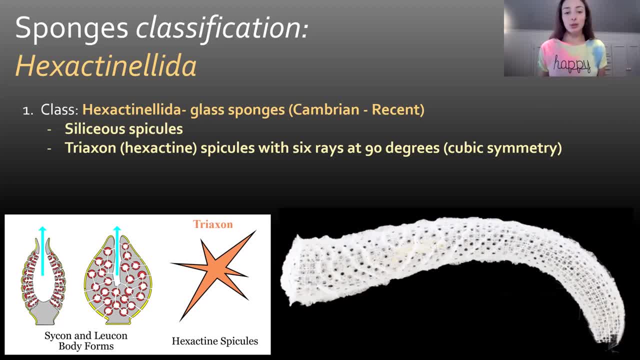 six rays at 90 degrees from each other, and this is also called cubic symmetry. And so we can see here at the bottom, this example of a glass sponge, very white and pristine, which is very different from the calcareous sponge, which is very white and pristine, and this is very different from the 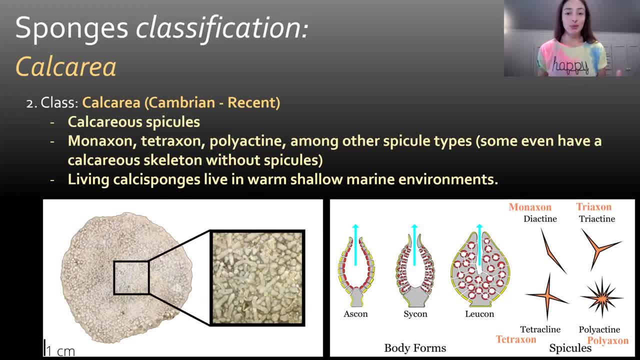 sponge fossils, which are going to be a bit more creamy colored, And so that's one way you can distinguish between siliceous and calcareous sponges without having to do any chemistry on them. So, moving to the class calcarea, we have the same time range- Cambrian to now- but we have 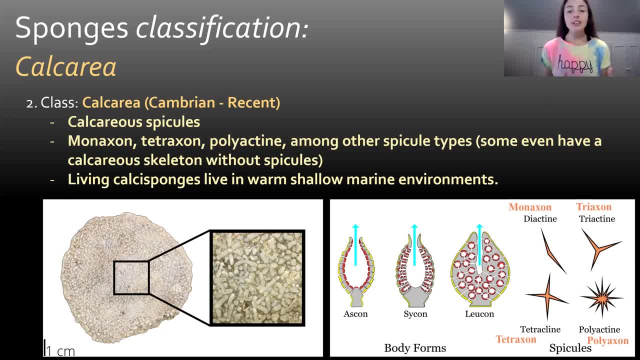 calcareous spicules instead of siliceous spicules, and their spicules can be a range of shapes. They don't just have to be triaxon hexactines, like the glass sponges do. They can be monaxon triaxon. 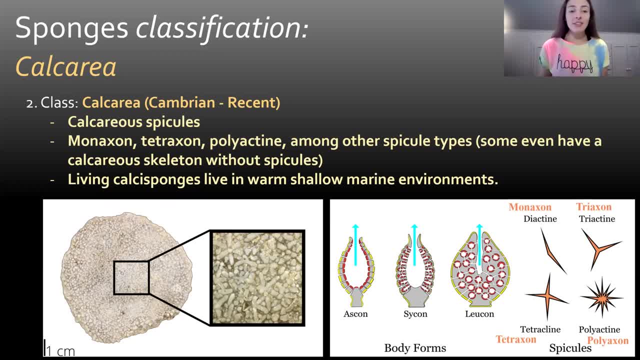 polyaxon- pretty much any shape you could want. Some even have calcareous skeletons without spicules. so they're very diverse. Now, before we move on, I do want to point out in the bottom right picture we have this sponge picture here. 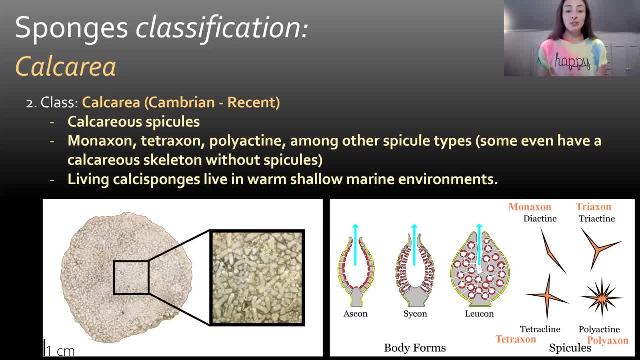 that I promised you we'd zoom in on so you could see all the spicules, And so we have this zoomed in square here showing their spicules and their shapes, and I highlighted a few of the star-like spicule structures in red here so you can kind of see them. And so if we go back and forth, you can. 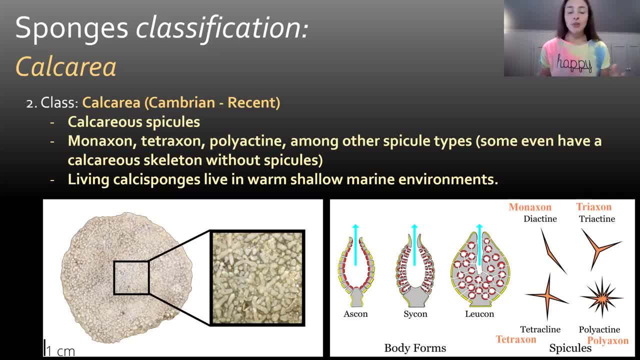 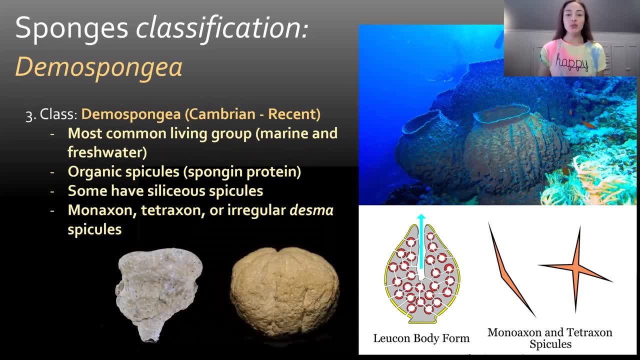 kind of see where the spicules are kind of in a structure. However, most of them are broken up, So there's a lot of broken up spicules. Moving on to demo spongia, these also lived from the Cambrian to now and they are the most common living group of sponges And they live in both. 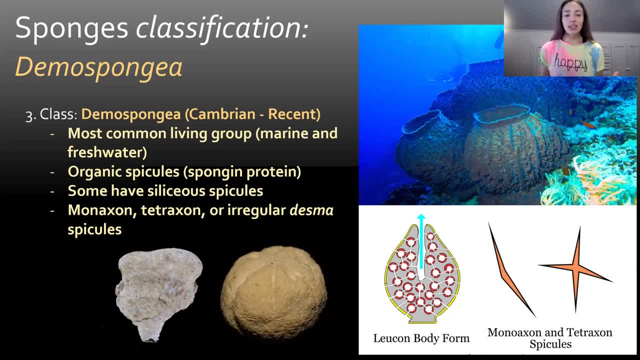 marine and freshwater environments. However, unfortunately, their fossil record isn't as complete as a lot of other siliceous and calcareous sponges, because they make their spicules out of the organic spongin material we talked about earlier, and these won't preserve. 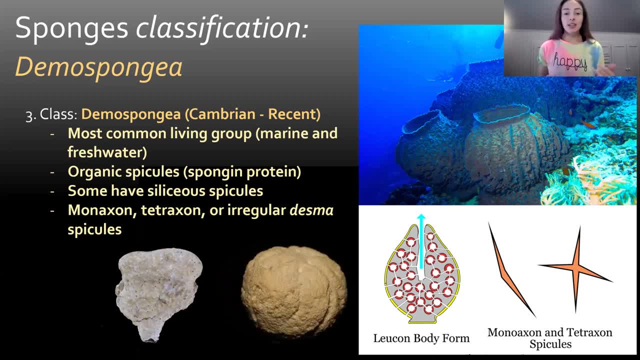 as often. However, in terms of type of spicule, they have monaxons and tetraaxons most common, and sometimes they have really irregularly shaped, knobby-like spicule structures called desmospicules, And this is more typical of organic spicules. You don't have the perfect of crystallized 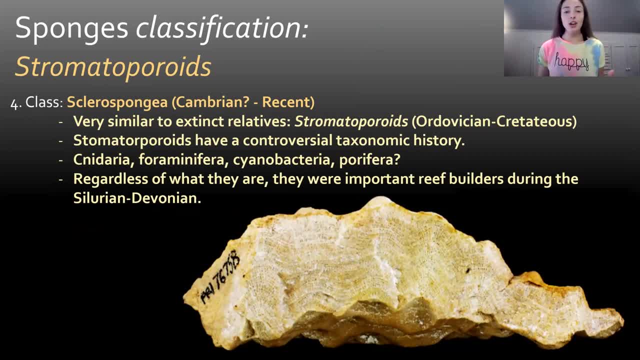 shapes because they're organic material, And the last class we'll talk about is the sclerospongia. Now I have it spelled right. This goes from the Cambrian to now, and I'll add to that possibly the Jurassic to now, And this is because some people think these stromatoporoids are part of. 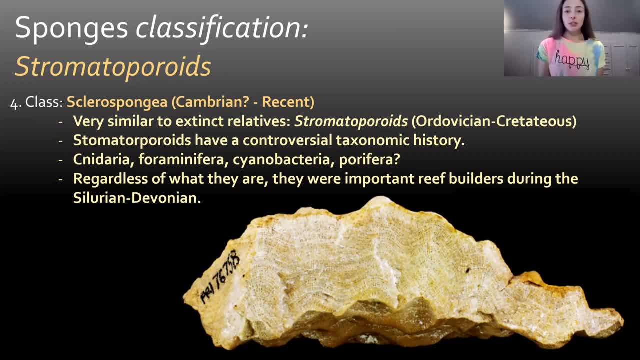 the sclerospongia and that the sclerospongia stromatoporoids are part of the stromatoporoids. The stromatoporoid sponges started in the Cambrian and some people think that the sclerospongia. 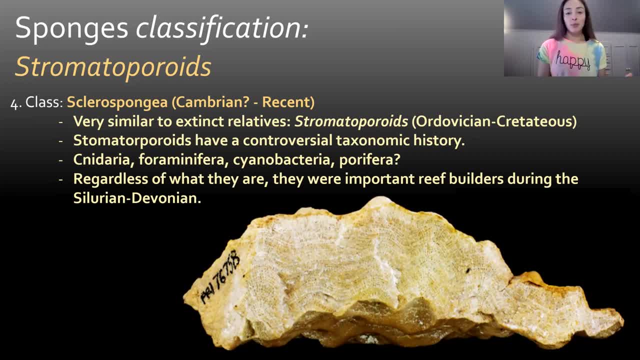 class doesn't start until the Jurassic and that stromatoporoids are just a distant relative. And some people put this class and the stromatoporoids completely in demospongias. and some people put the stromatoporoids in with the Cnidaria Foraminifera or Cyanobacteria. So this is 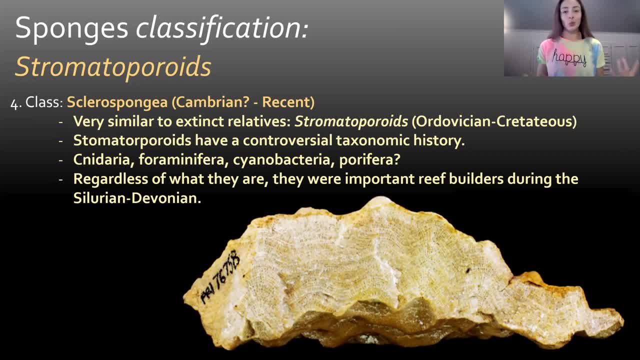 just a really crazy taxonomically confusing situation for the sponges here. But we're going to try and just talk about stromatoporoids, Explain how important they are and a little bit about their structure, and maybe that will at least. 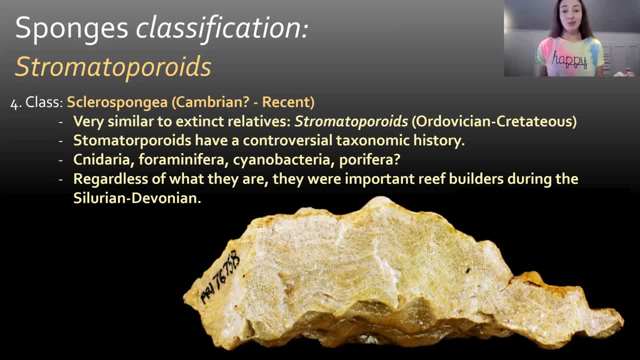 a little bit help you in your class. Sorry, I can't be of more help in terms of the systematics of this group. So, in terms of stromatoporoids, they have a time range from the Ordovician to the Cretaceous. 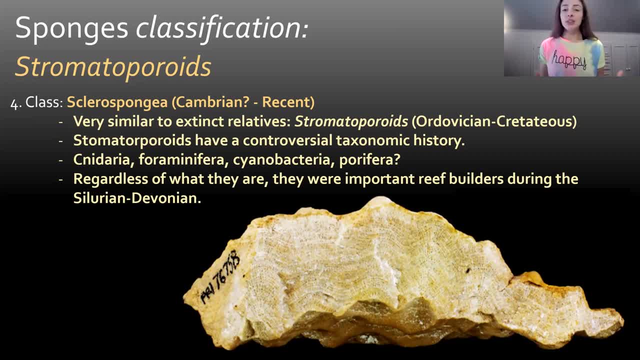 So they are completely extinct, but they are really interesting fossils and have a very distinct morphology. This is why they're so hard to place. They have features similar to Periphera, but they lack spicules, which is why a lot of people put them in with Cnidaria. They also have this layered. 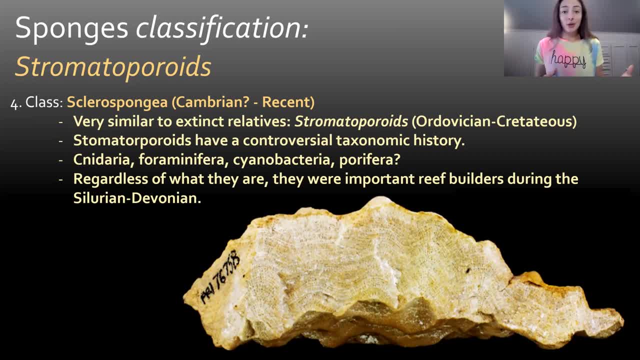 wavy structure which makes them similar to bacterial mats like Cyanobacterial stromatolites, and they also have been thought to be similar to Foraminifera. So these have very distinctive features that just can't be placed very easily. But regardless of what they are, they were very 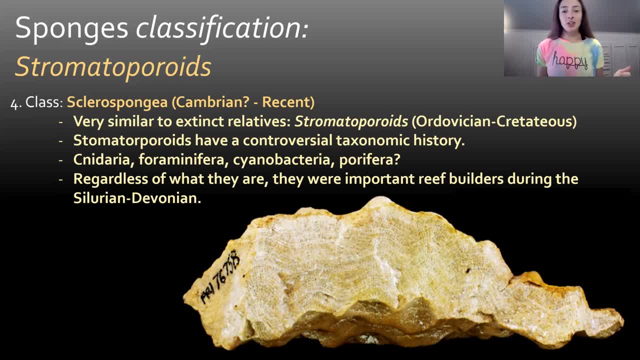 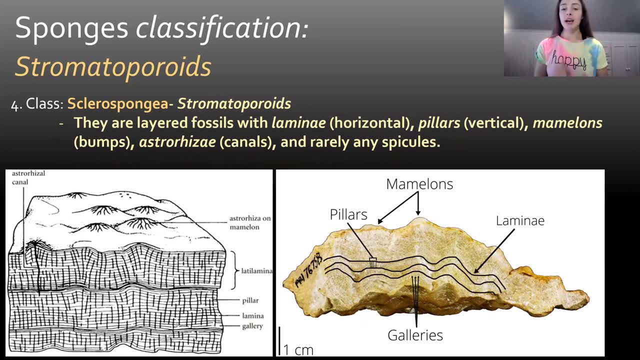 important reef builders for a lot of the Paleozoic, namely in the Silurian and Devonian. As we can see in the picture below, we have this specimen where we can see these wavy layers shown in the black lines. now, and these wavy layers are pointed out here as being called 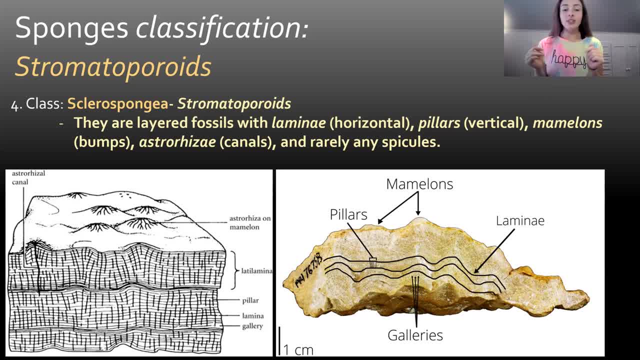 laminae. And then we have vertical lines within these layers- shown on both these pictures- the sketch diagram as well as the real fossil picture, and these vertical sections in between the layers, or the laminae, are called pillars. And then we have these bumps on top because of the waviness. 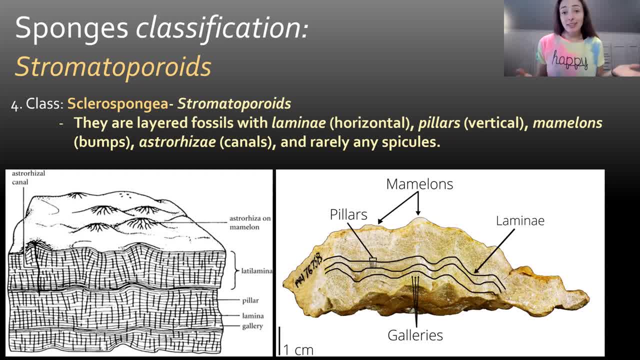 of the stromatoperoid and these bumps are mammillons- I think I'm saying that right. And then they have a star-like pattern of canals that go through the mammillon bumps, and these are shown in the left side of the left image. and these are the stromatoperoids. And then we have these: 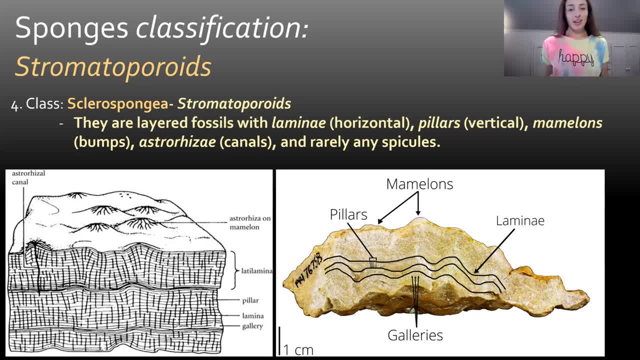 these are called astro- astrorhizae, Astro-. I should practice saying these things before I start these Astrorhizae. Okay, we're gonna go with that: Astrorhizae, Astrorhizae And, as we can see, the last thing I. 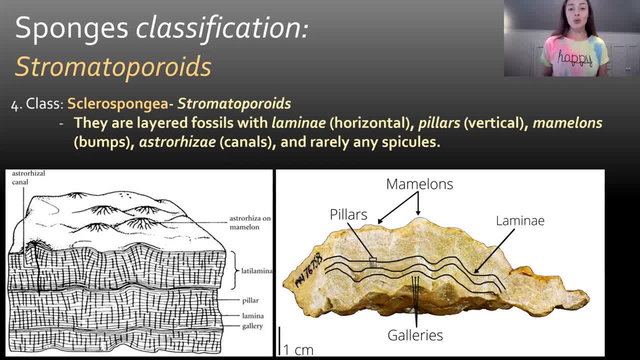 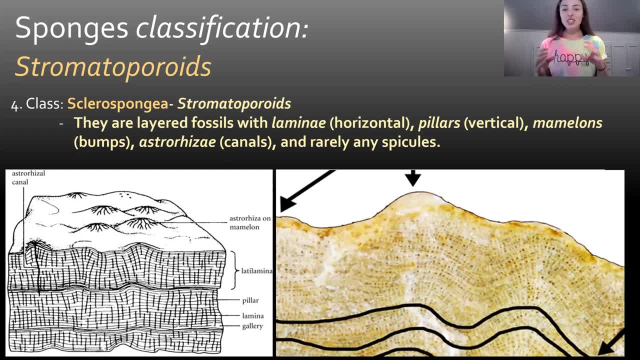 mentioned is that they rarely contain spicules, which is one of the reasons they were so hard to place in terms of classification. Before we move on, I want to zoom in on this picture to the right so that we can see just the amount of detail that these laminae and pillars and canals, and 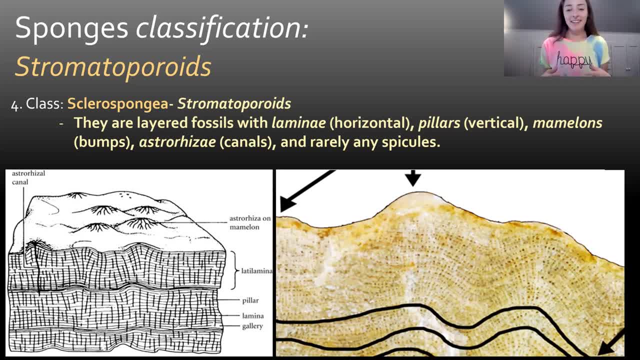 galleries or the spaces in between them have, And so we can see in this image that all the laminae and pillars are very fine, delicate structures that are very, very distinct, And so this is super cool to find, and you'll immediately 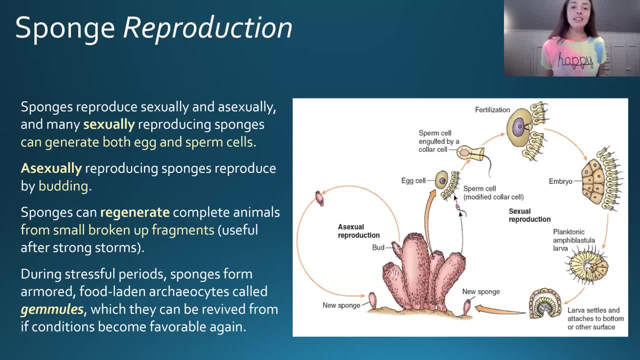 know what it is. if you find this kind of pattern in a rock, you pick up And, like we said, the last group that we would talk about for this lecture is the archaeocyanthids. However, we're going to talk a little bit about sponge reproduction, sponge ecology and sponge evolution before we get to. 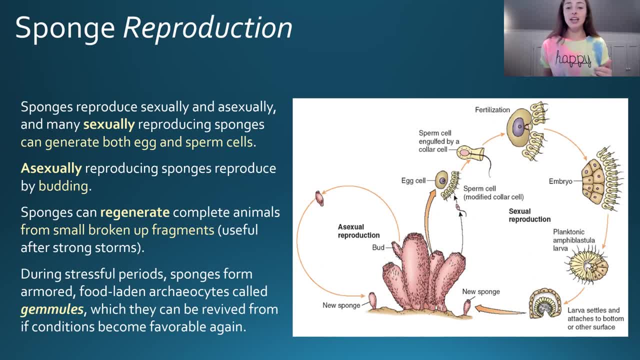 that, And so on this slide we can see that in the figure to the right we have this diagram showing sponges producing both egg cells and sperm cells, Because they can produce both of these. they can reproduce sexually with these egg and sperm cells, which eventually form into larva. 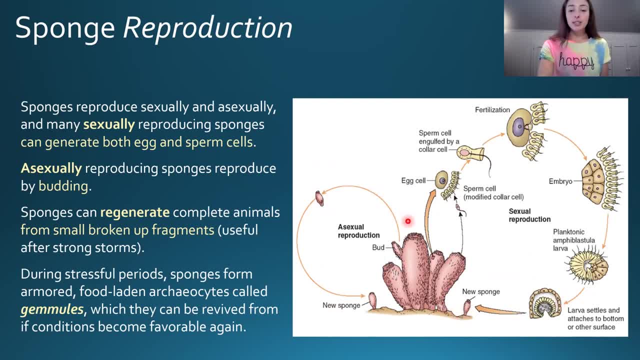 which will form a new sponge. However, they can also reproduce asexually through budding from pre-existing sponges. Additionally, sponges can regenerate complete animals from just broken up fragments of a pre-existing sponge, And this is very useful for sponges because a lot of times, 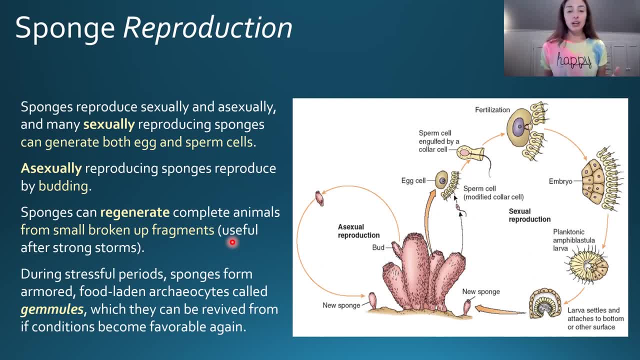 after really strong storms, if they're living in a really shallow marine environment, they can be broken up like crazy by the waves, And then they can later regenerate themselves to become an entire animal again. Another really cool thing that sponges can do is to form into gimules. 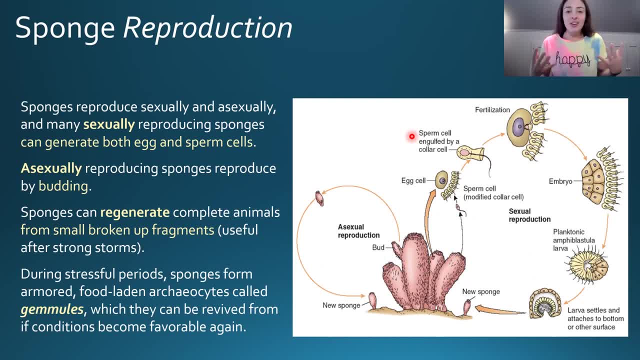 which are just little armored nodules of food-laden archaeocytes that can basically protect the sponge in a stressful or nutrient-poor area or period in time until that sponge's environment becomes favorable again, And then it can revive itself, which is insane to me. 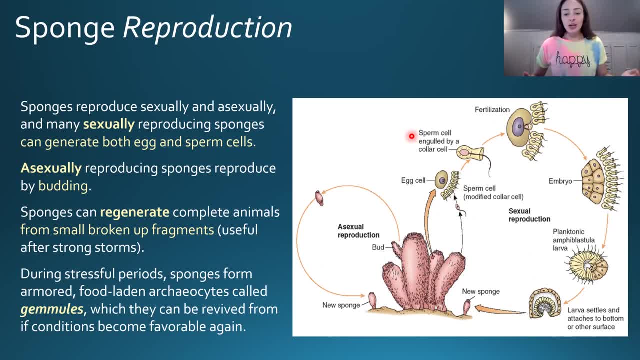 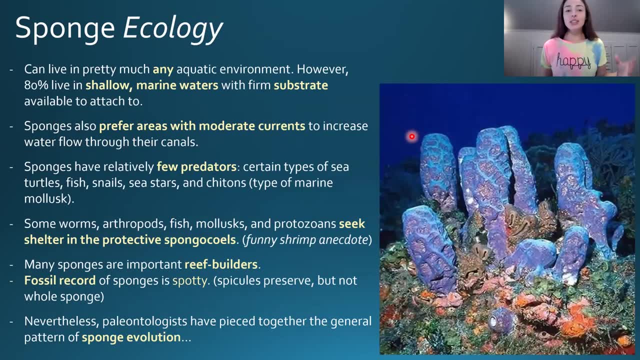 I mean, could you imagine if we just like go into a pod when you know we don't have enough food available to us and then come back out when we do? So these guys are pretty awesome that they can do that In terms of where they live, even though they can live in pretty much any aquatic. 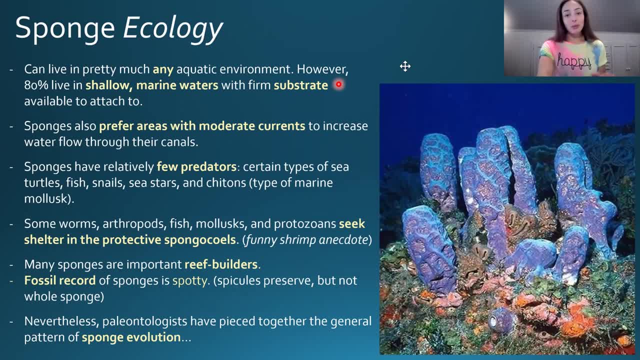 environment on Earth today. the majority, or about 80% of them, live in shallow marine waters, where there is substrate available for them to attach to. Also, they prefer areas with moderate to strong currents, because this increases the water flow through their canals, and so they can. 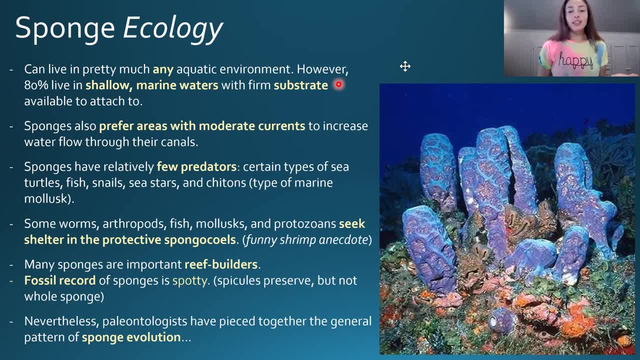 filter feed easier. And another beneficial thing for sponges is that they have relatively few predators. Basically, certain types of sea turtles, fish, snails, sea stars and chitons might munch on them from time to time, but the most thing they're useful for is for protection. 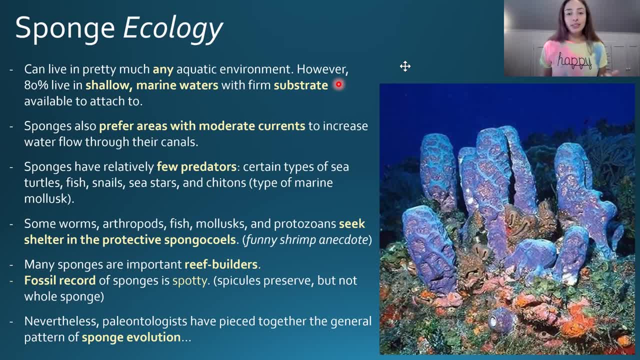 Some types of worms, arthropods, fish, mollusks and protozoans seek shelter in their protective spongicles, And so I put here to remind myself, Funny Shrimp Anecdote. That's because the book that I'm reading that is helping me make these lectures, which is linked below if you want to. look into. it is called Funny Shrimp Anecdote, And it's a book that I'm reading that is helping me make these lectures, which is linked below if you want to look into it, And so I put here to remind myself. 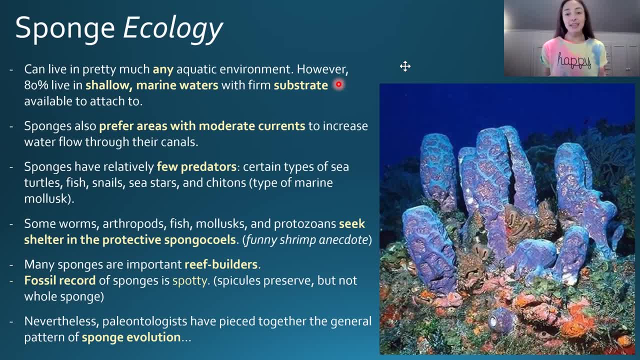 Funny Shrimp Anecdote. That's because the book that I'm reading that is helping me make these lectures they explain this in a really funny way, or I thought it was funny. But basically they mention that sometimes when shrimp go in to the spongicles for protection, they stay in there. 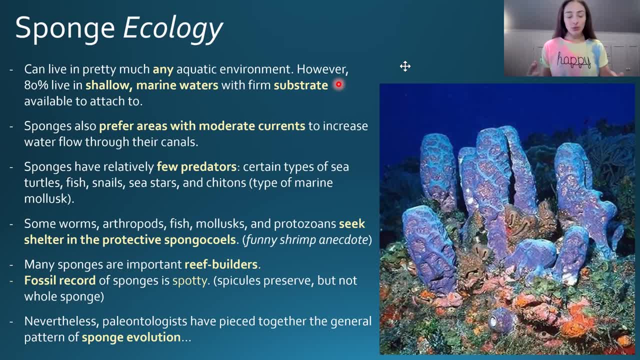 so long and molt a bunch of times, because shrimp molt to grow that they get so big by the time they try and go out. they can't fit out of the spongicle And so they are stuck in there, And sometimes when pairs of shrimp get stuck in the spongicle they can get fossilized like that. 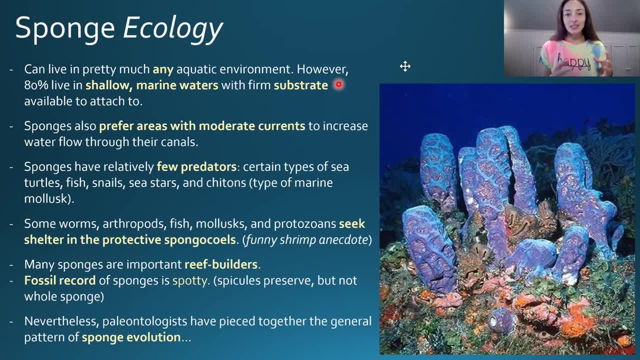 And these fossilized shrimp pairs that are strapped in this glass ball are actually a common wedding gift in some cultures, because apparently the concept of these two shrimp being trapped inside this ball is symbolic of marriage. I just thought that was hilarious, So anyway. 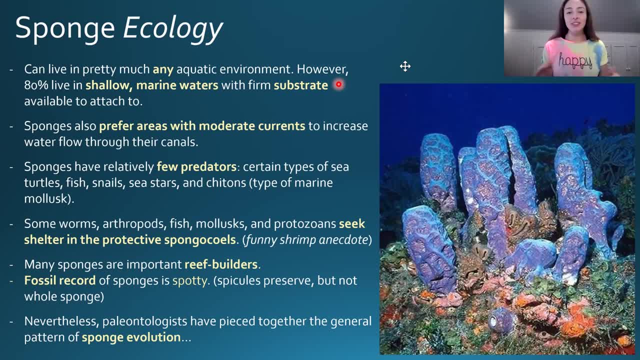 moving on. Many sponges are important reef builders and we'll talk about kind of the history of different sponges being dominant in reefs at different times in our history on the next slide. But the fossil record is a little fuzzy for sponges because, like we said, the 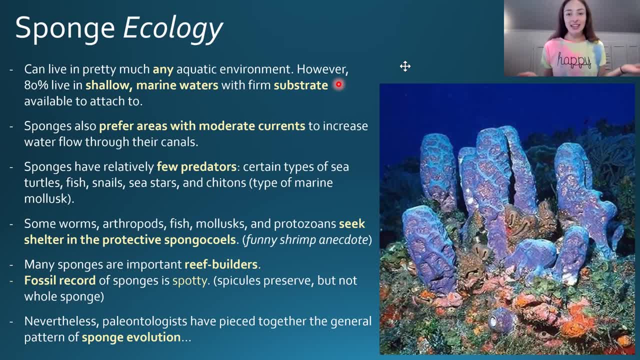 spicules preserve, but sometimes they're just spicules, They're not actually attached to a sponge animal in a fossil, And so, because the whole thing is about the fossil record- sponge doesn't always preserve- we have had to piece together a general pattern of sponge. 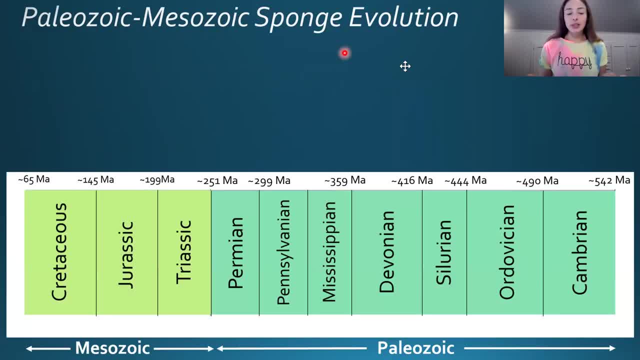 evolution without an entire picture, And so with this we'll look now at the evolution of sponges. So if we look here at this timeline from the Mesozoic-Paleozoic, first, we have the sponge classes all evolve, We have the Hexactanilids, the Calcaria, the Demosfungia. 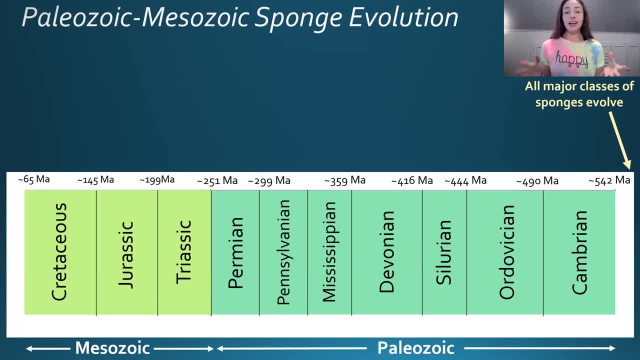 and the Sclerospongia- maybe question mark- all evolve here in the early Cambrian, Then what we have is the extinction of the Archaeosciathans, which I know we haven't talked about but I'm going to. But I thought for the purpose of the evolutionary slide I should include it on this. 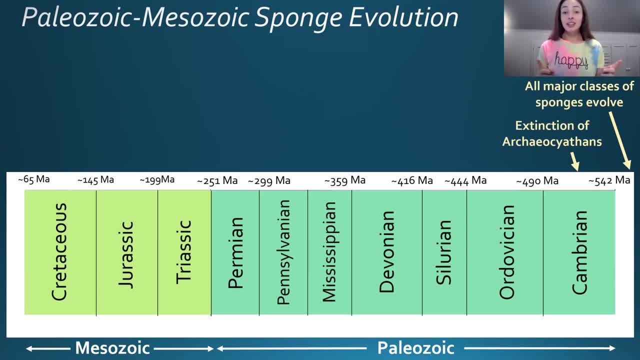 timeline, because the Archaeosciathans were really important refielders and nothing in the early to middle Cambrian was creating reefs other than Archaeosciathans, And so, after their extinction, other types of refielders or types of sponges that could refield started to evolve. So then, 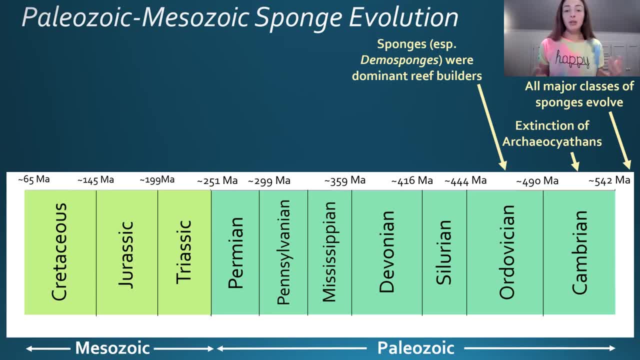 we have the sponges, especially Demosfungia, become dominant refielders in the Ordovician, And then we have tabulate and rugose corals diversify and kind of get into the refielding business as well, And then we had sponges become less important refielders because of coral. 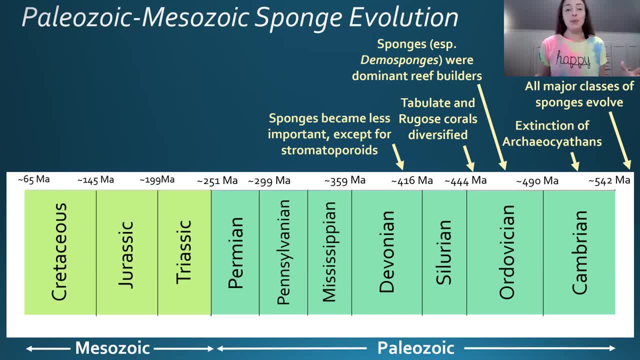 evolution and corals taking over the reef building business, if you will. However, one of the groups that didn't become less important in reefs was stromatoporoids- Coral strome reefs were really common around this time. Then you had the Doponian extinction, which caused a decline in coral. 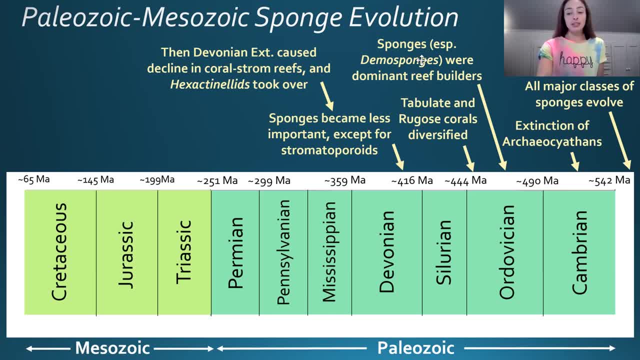 strome reefs And Hexactanilids actually took over the reef building business, which, if you remember, are the glass sponges. And then you had Permian reefs, which were largely built by calcareous sphincterzoan sponges. Then you had the Permian extinction which, thankfully, all of the 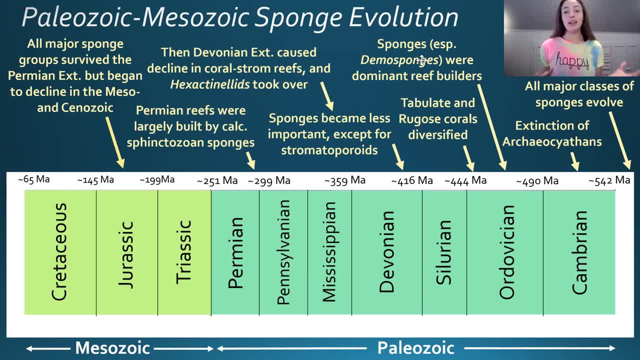 major sponge groups did survive. However, during the Mesozoic they began to decline in their dominance And at the end of the Mesozoic, stromatoporoids went extinct at the K-T extinction boundary. And during the Cenozoic all the major sponge groups continued to decline in. 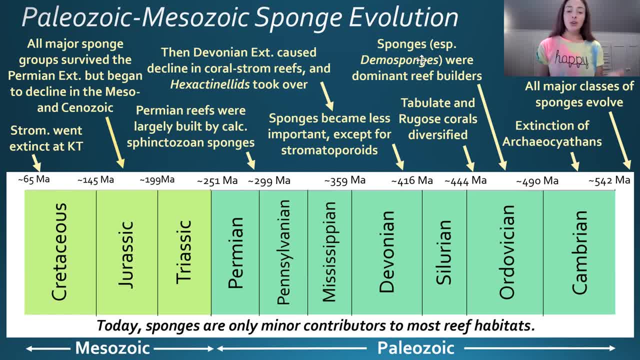 their abundance and dominance to the point that today they are only minor contributors to most reef habitats. However, they're still very common on Earth. today, You just don't see them building huge reefs. Now, finally, moving on to the Archaeocytathans, Archaeocytatha is a group of 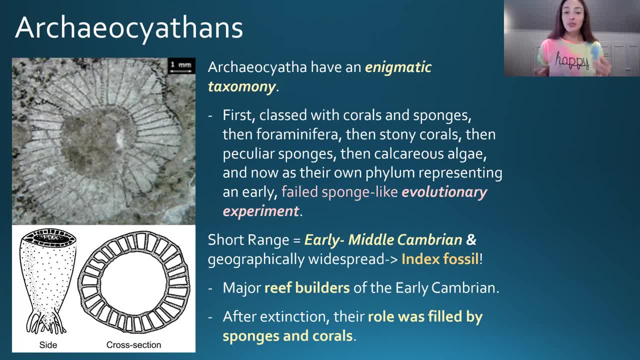 sponge-like animals with a very enigmatic taxonomy, which we already discussed, And because of this, paleontologists have tried placing them in with corals, sponges, foraminifera, stony corals, peculiar sponges and even algae. However, now paleontologists lean toward them being some sort 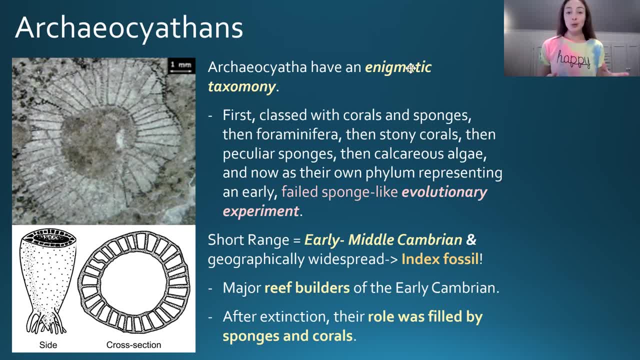 of failed sponge-like evolutionary experiment, So that's what we're going to treat them. as for this video, Archaeocytathans had a very short time range. They only lived from the early to middle Cambrian period, which is the only the first period in the Paleozoic. However, they weren't this just. 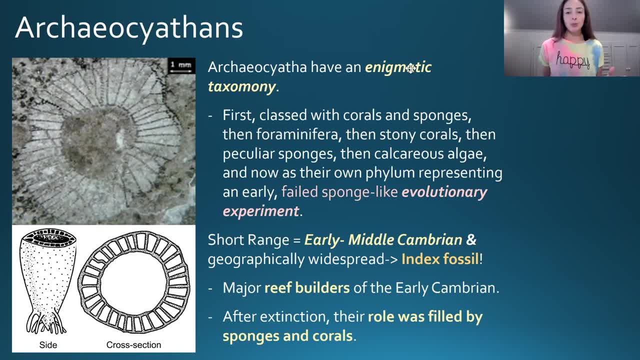 measly unsuccessful experiment. They were incredibly geographically widespread to the point where they had global dominance in terms of reef building. And because of this widespread of Archaeocytathans they make wonderful index fossils And so we can correlate Cambrian period. 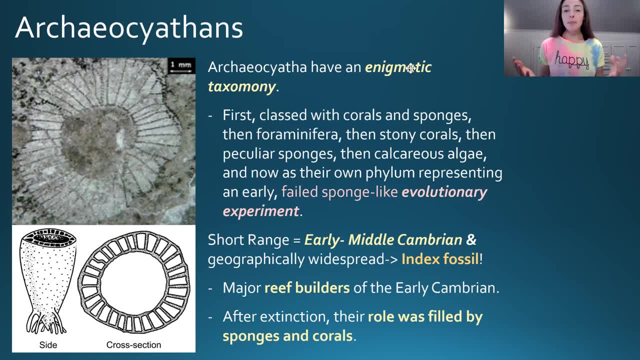 sections across the globe with these fossils. However, their complete success during their lifetime makes it really difficult for them to survive. So we're going to take a look at some of the fossils that were found in the middle Cambrian period, and we're going to take a look at some of 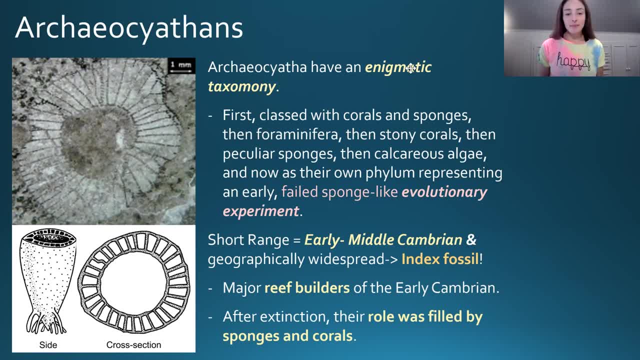 the fossils that were found in the middle Cambrian period, and we're going to take a look at some of why they came to an abrupt end in the middle Cambrian, And so this is a very confusing thing, and it's something that I think is really cool to look into. So if you want to look into, 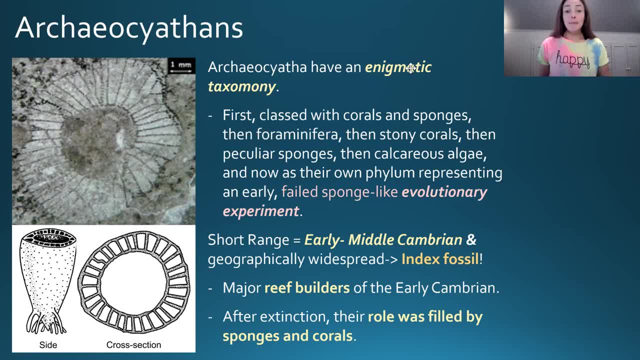 Archaeocytathans and trying to figure out what happened in the middle Cambrian that made them go extinct so abruptly even though they were so happily dominating the world. that would be a really cool thing to go into. So just a thought. And then, after their extinction, their role was: 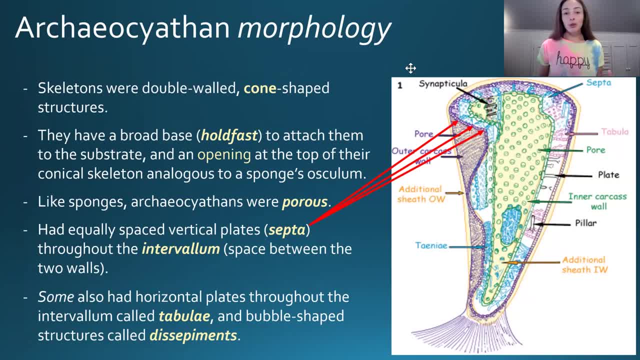 filled by sponges and corals. To get into a little bit of their morphological characteristics, they had pretty simple corals. They had a lot of corals, They had a lot of corals, They had a lot of corals. 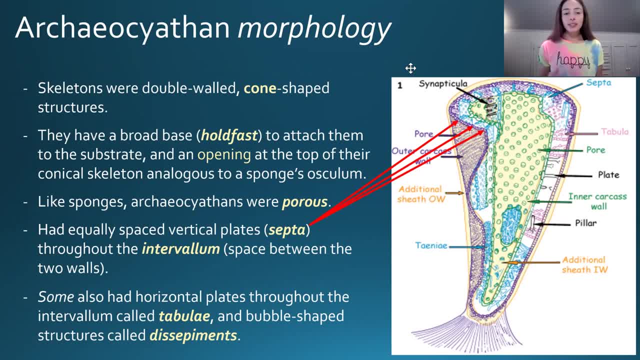 They had cone-shaped structures shown here in this picture. They have a holdfast at the base to attach them to their substrate and they have an opening at the top of their skeleton, similar to a sponge's osculum And also like sponges. they were very porous. However, similarly to 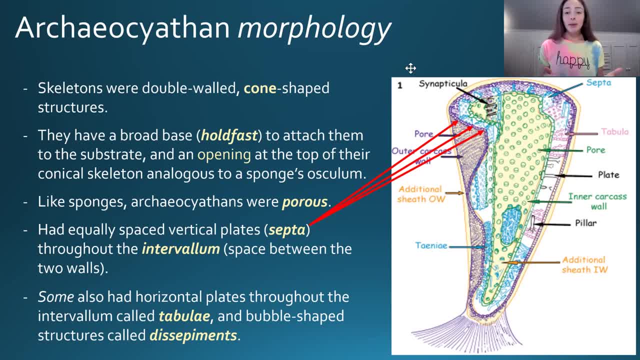 cnidarians or corals, which we'll talk about next time. they had septa, which were vertical plates equally spaced throughout the space in between their two walls in their structure, And this space is called their intervalum. Additionally, they had horizontal plates. 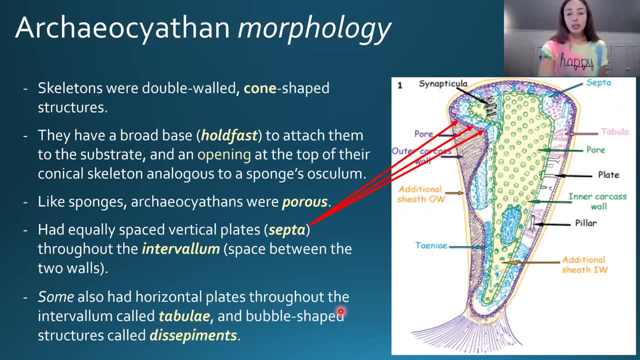 called tabula, or plural tabulae, and bubble-shaped structures, also in their intervalum, called decepaments, And these are all characteristics shared with tabulae and rugose corals, and we'll talk about those in the cnidarian video. But these similarities to sponges and cnidarians both made 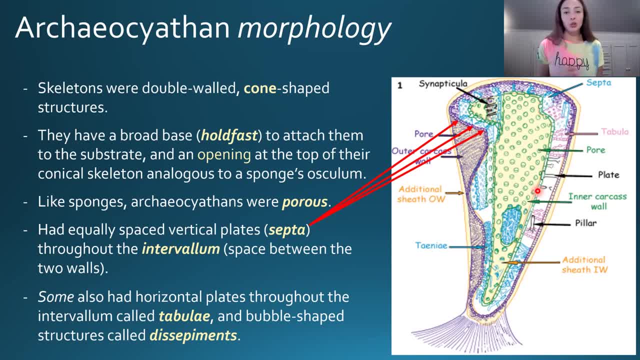 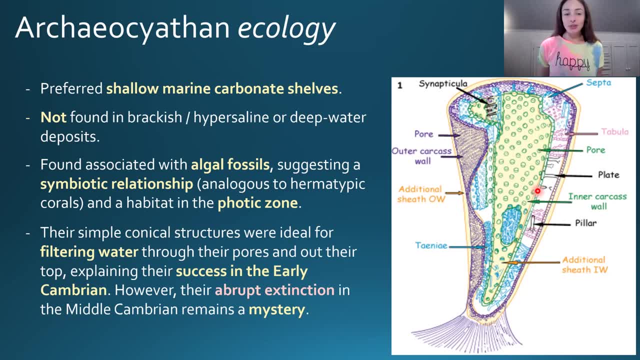 them so hard to place and is why we consider them a whole different group. In terms of ecology, the Archaeosciathans preferred shallow marine carbonate shelves, and this makes sense if they were refielders, and they were not really found in Brachycephalae. 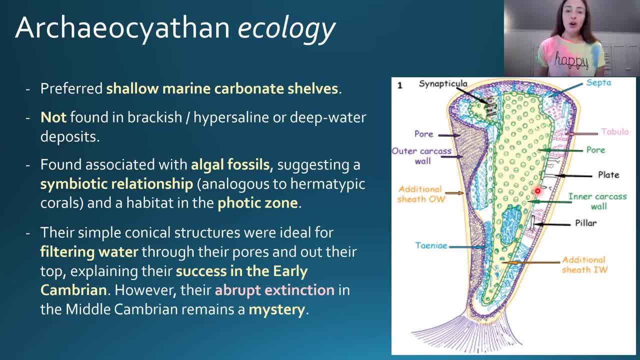 They were for Uranian sandstone, andichaea wateratic, PhDs, whichbia canolae, And they were always associated with algae fossils when they were found in the Rock Record, so this suggests an interesting symbiotic relationship between them and algae. Here's an example of these bird: seashells. 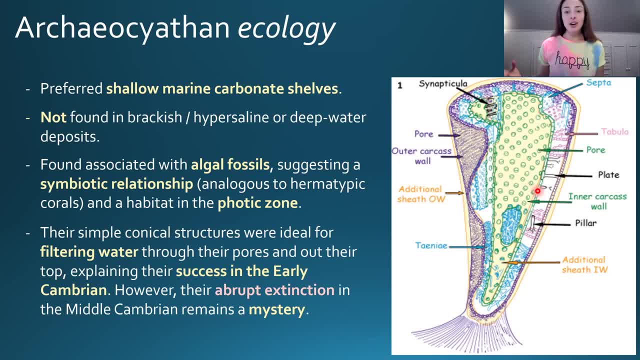 Serin tales and♡ Yeahah. so this analogy is fairly true- that encounters with algae are pileups and they can Chop比 also FX c ri o i ze algae and archaeocyathins in the Cambrian, and this may have been the first time that that kind 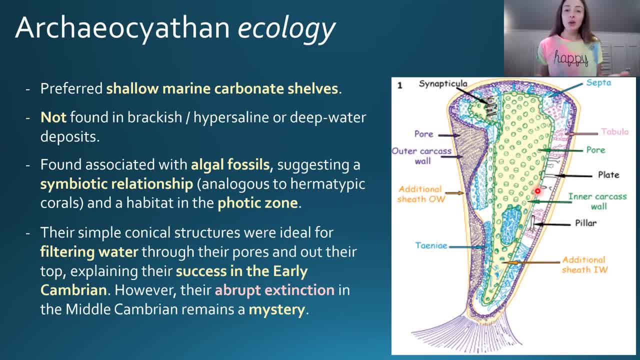 of relationship evolved, but we don't know for sure. This is speculation based on what they're found with in the fossil record. However, what it does tell us for certain is that the archaeocyathins like to live in the photic zone because the algae fossils they're found with also needed to live in. 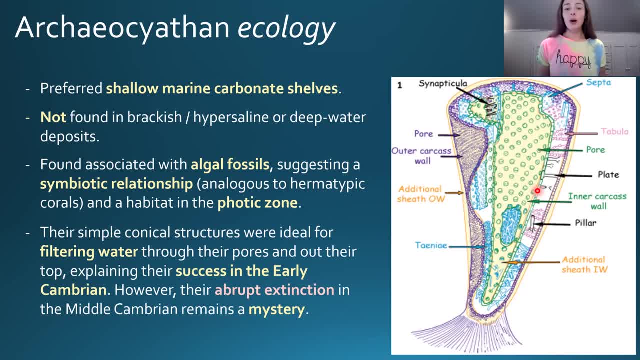 the photic zone to get sunlight. Additionally, their simple conical structures were ideal for filter feeding, just like sponges and corals through their pores and out their osculum. This beneficial conical structure for filter feeding explains their success in the early Cambrian. but 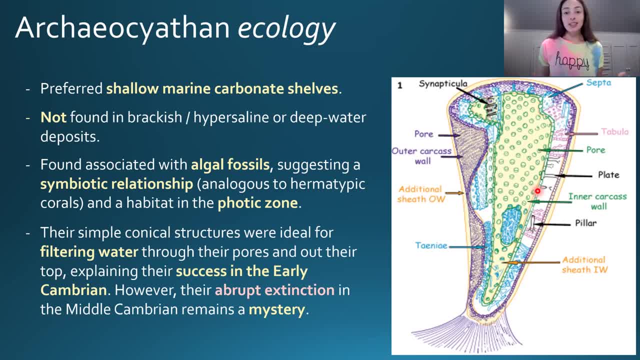 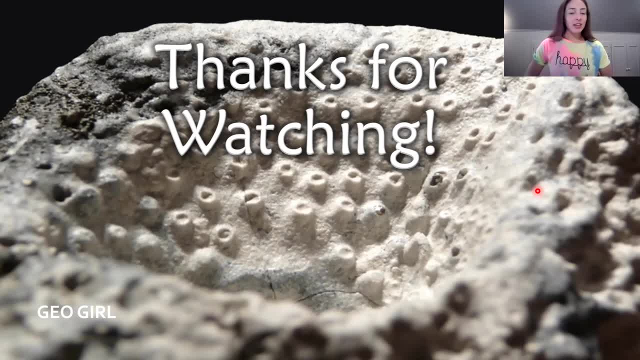 it doesn't explain their abrupt extinction And, like I said, this remains a mystery. So I hope that you find that as cool as I do, and I hope that you're excited by the fact that we don't know every single thing about different phyla and their evolution throughout Earth's history, and I hope